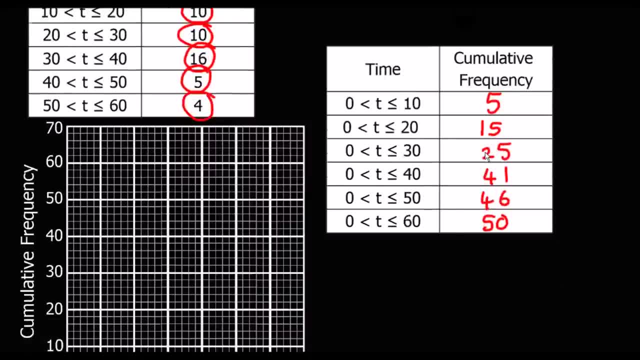 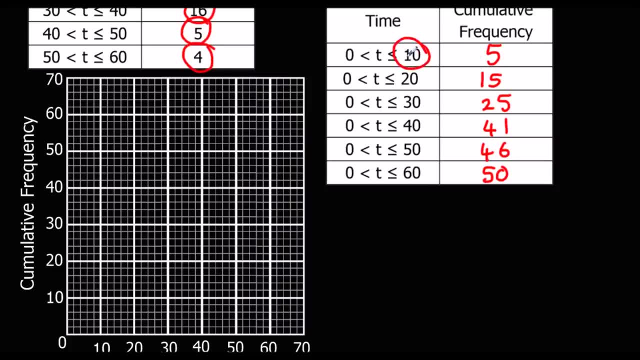 along. That's our running total. So when we're asked to plot the cumulative frequency graph, this is up to 10.. This 5 is up to 10.. So we're plotting this top number. We don't plot the midpoint because there haven't been 5 by the time we get halfway. There's only been 5 by. 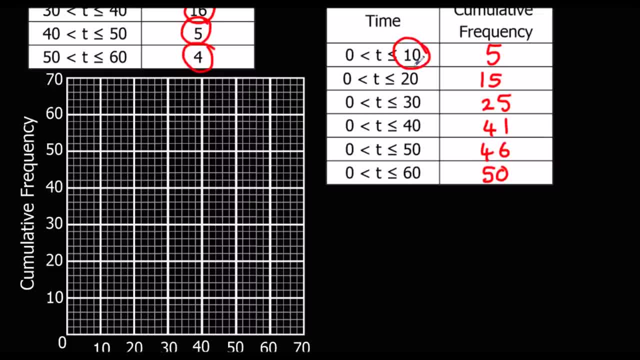 the time we get to 10.. So we're plotting top point: cumulative frequency. So these are the points we want to plot. So we're plotting 10 against 5 on cumulative frequency. So that's in the middle there, 20, 15.. So 15 should be in there, 30 against 25.. 40 against 41.. 50 against 46.. And 60 against 50.. 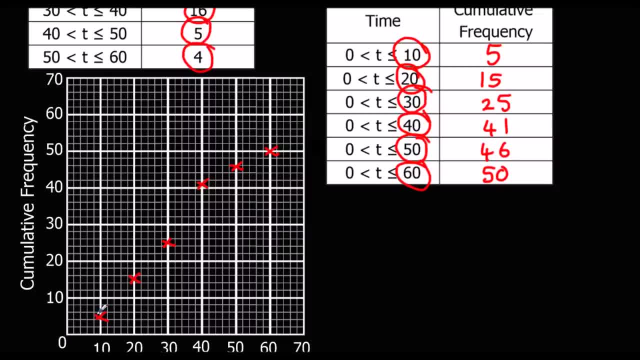 And then when we join them up, it should be a smooth curve, So a curve that joins up all these points. So hopefully I won't mess this up, I've missed a point there, But we want to join up the smoothest curve we possibly can. Then they could ask us questions like finding the median from. 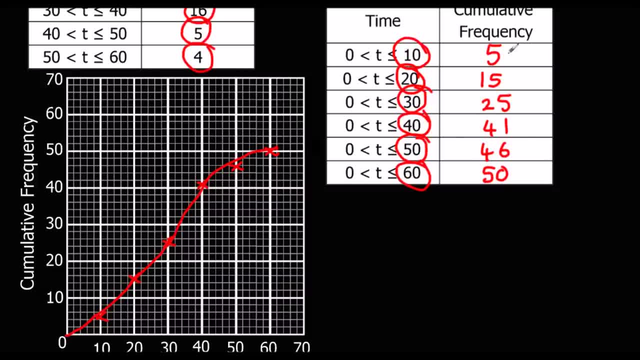 here. So if there's 50 people, 50 numbers in our on our graph, the median is going to be 50. So the median is halfway. So the median would be 25.. So what we'd be looking for is 25th person. 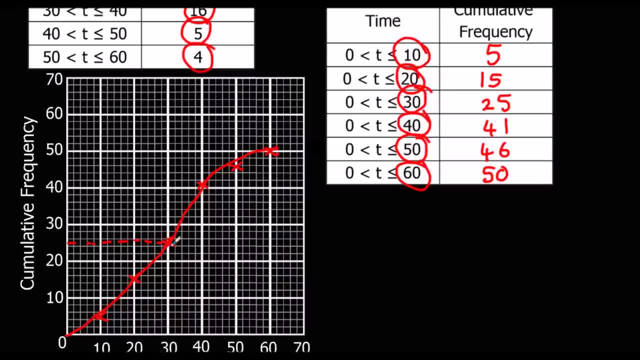 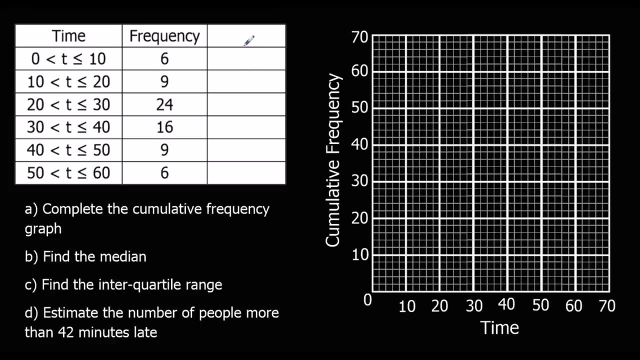 We'll go along to there and go down. So the median in this case is 30.. Let's have a look at a different one. So here it's presented differently, but we're still going to do the same thing. Cumulative frequency is still a running total, So we'll put cumulative frequency. 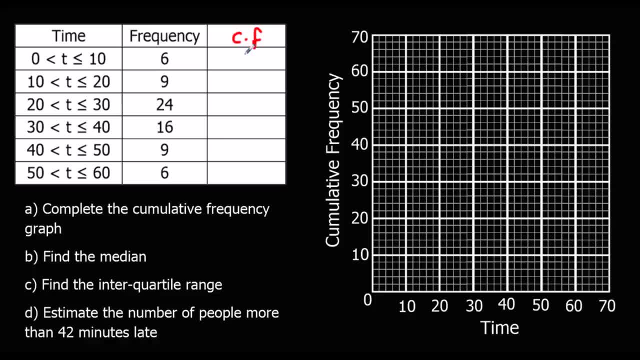 in this box And we're going to add them up as we go along. So 6.. And then we're going to add on the next one. So 6 plus 9 makes 15.. Plus 24 makes 39.. Plus 16, 55.. Plus 9,, 61.. No 64.. Plus 6,, 70.. 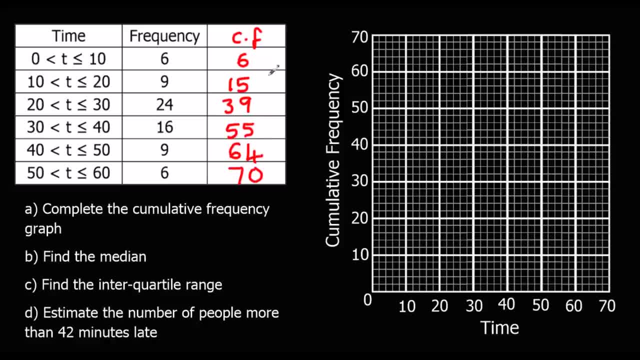 So these numbers are up to 70. And when we plot them we're going to plot top point against cumulative frequency, Always the top point. So 10 against 6.. So 10 goes with 6.. 20, 15.. 30,, 39. 40,, 55. 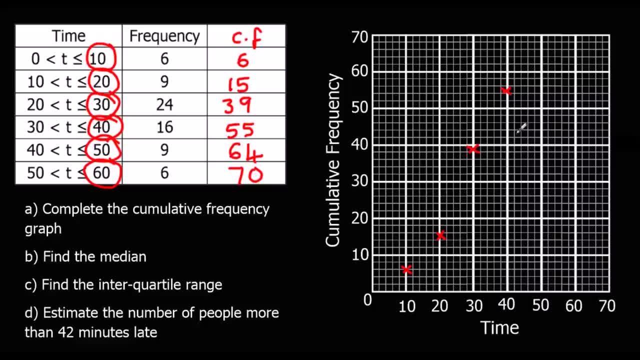 50 goes with 64. Up there, And 60 goes with 70. And then we join them up again with a smooth curve. So up like that And a smooth curve joining all the points. So then we're asked to find the median. 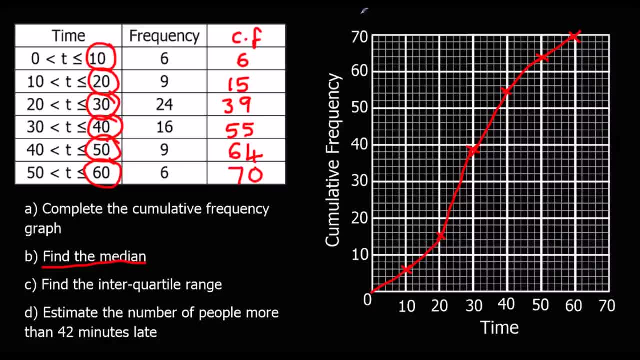 If there's 70 people, if there's 70 on the frequency 70, we want halfway, which is 35. So, again with a ruler: if we can go from 30.. That's 30. Go from 35 across and down from there. 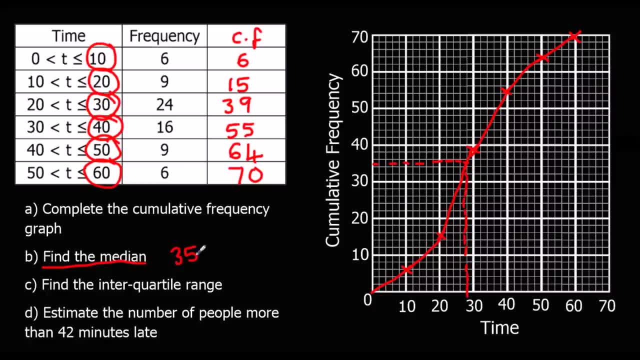 So that comes out as 28 seconds. So this isn't the answer. So that's what we've been looking for And the answer is 28 seconds: The interquartile range, So the upper quartile and lower quartile. 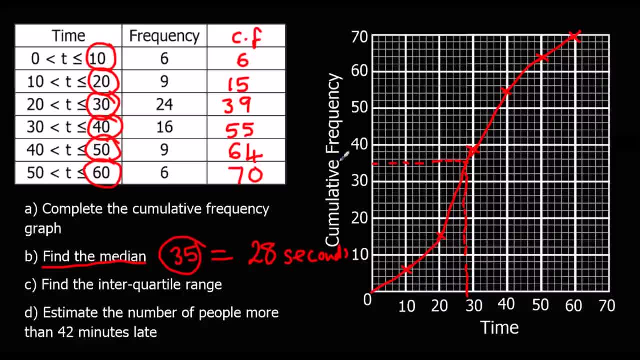 The median's half the data, which was the 35th piece. So the quarters are well. so we only go. one quarter of 70 is half of this, So 17.5.. Just underneath 18.. So we go just underneath 18 to the line. 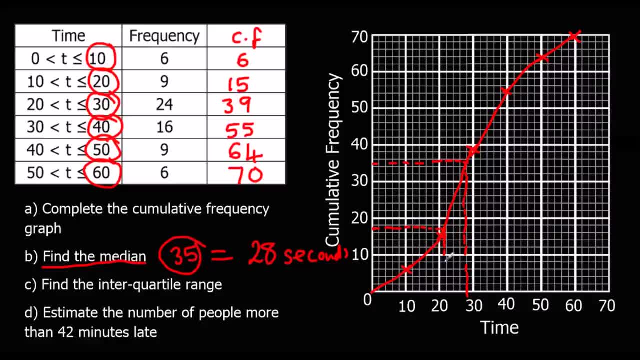 And down from there, which is well 21 or 22 seconds. So let's say lower quartile is 22 seconds, Upper quartile so three quarters of 70. So that'd be 17.5.. 17.5 plus 35. That would be 52.5.. 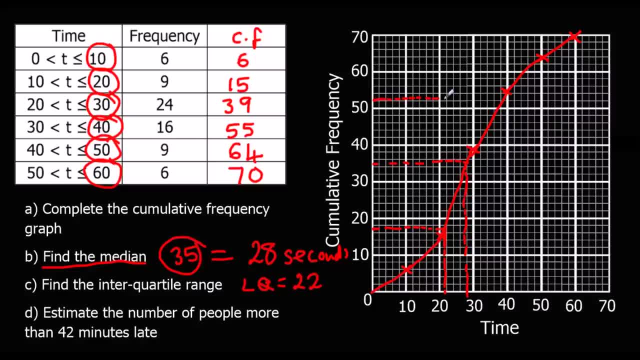 So just above the 52. And then from there we go down. Let's say that's in the middle, So that would be 39. So the upper quartile: 39 seconds. So the interquartile range: 39.. 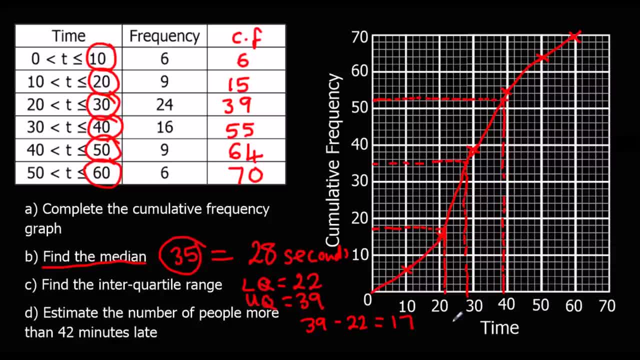 Take away 22. And that is 17. 17 seconds. Usually you'll find that these numbers are actually easier, And it's normally 80. So a quarter would be 20. Or 100.. A quarter would be 25.. 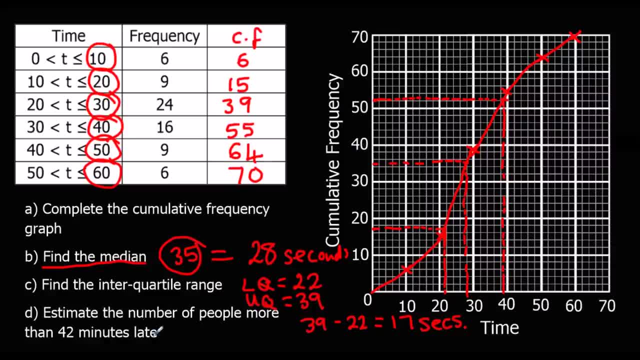 They're not usually 70.. Estimate the number of people more than 42 minutes late. So these were actually minutes. Let's change them to minutes. So the number of people More than 42 minutes late. So we're looking at 42 minutes. 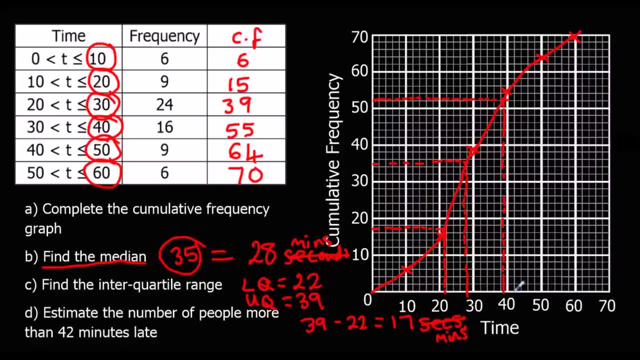 Which is here, Go up to the curve All the way along that line And it comes out there. So it's coming out at 56.. So, 56. Um Is So it's coming out at 56.. 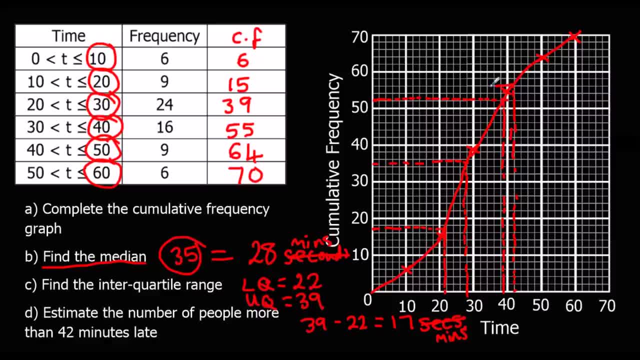 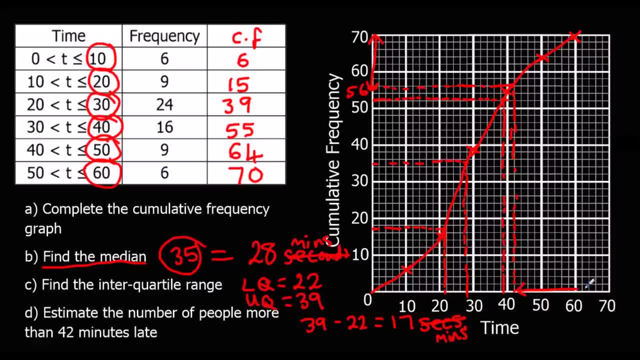 Is Is Is. Well, After 42 minutes, 56 people have arrived. So we're looking at the gap here. More than So, more than 42. It's this side, So It's: How many more than 56 have we got? 56 have arrived. 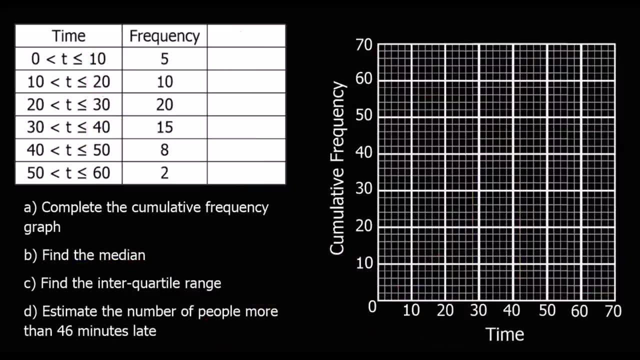 How many more of? we got So 14.. Okay, So, first step to get a running total, so cumulative frequency, a running total 5, add on the next one, keep adding on the next one: 50,, 58,, 60, so a much nicer number this time. 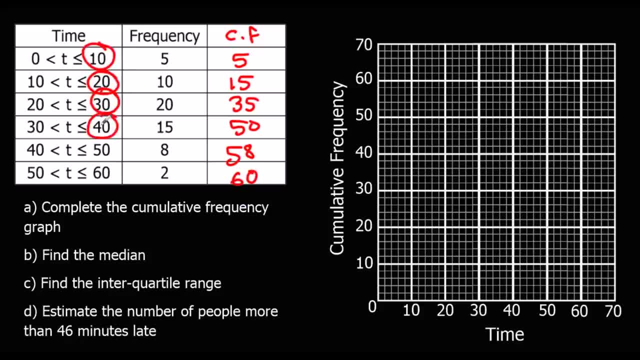 Take the graph, plot the top points. top points against cumulative frequency. so 10 against 5,, 20 against 15,, 30 against 35,, 40 against 50,, 50 against 58, and 60 against 60.. 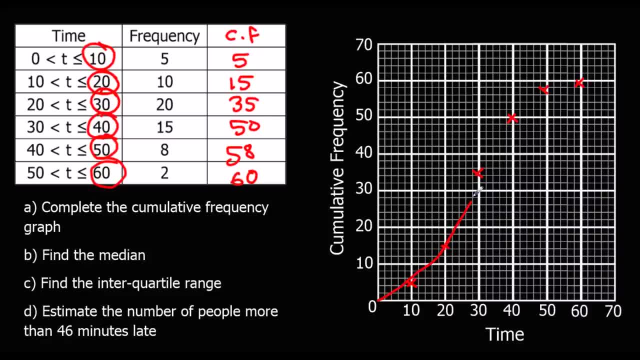 Smooth curve to join them up. Try and not miss the point Points, like me. And then we're asked to find the median. so the median's a middle number. If I've got 60 on the frequency, 60, half of that the 30th, so the 30th one along. 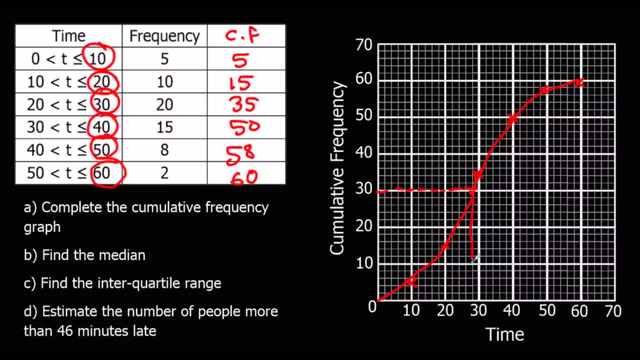 from 30 and down, so 28,. 28 minutes Interquartile range. so we need the upper quartile and the lower quartile. So a quarter of 60 is 15, so we go along from 15 and down. so that was 20.. 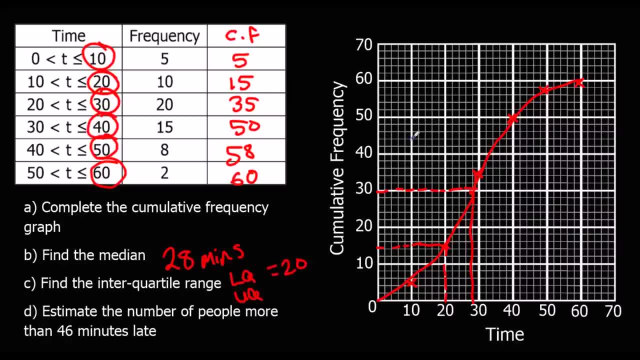 Upper quartile, that's 45. So along from 45 and down, so halfway in there, That's 37. So 37.. Interquartile range: 37. Take 20.. We'll keep going. 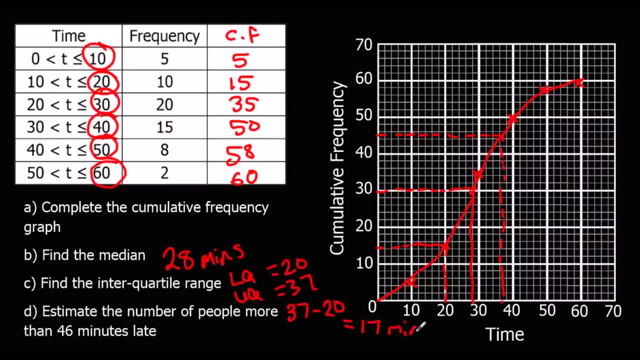 Okay is 17 minutes. number people more than 46 minutes late, so we're looking at 46 on the minutes up from there meets there in the middle and that's going to come out at 55 people. so 55 there was it more or less than it was more than so we want. 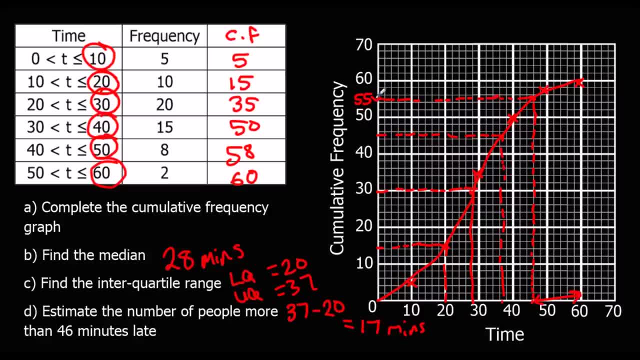 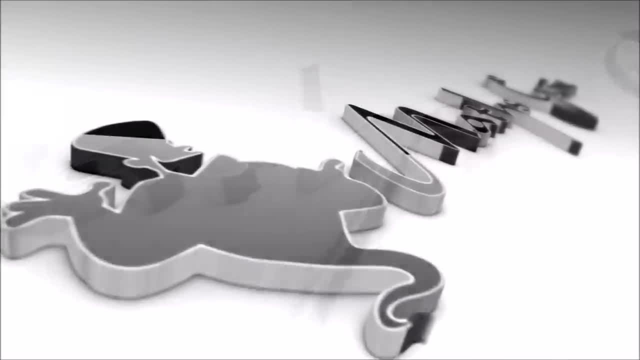 those people, which are those people? that's five people, five people you.